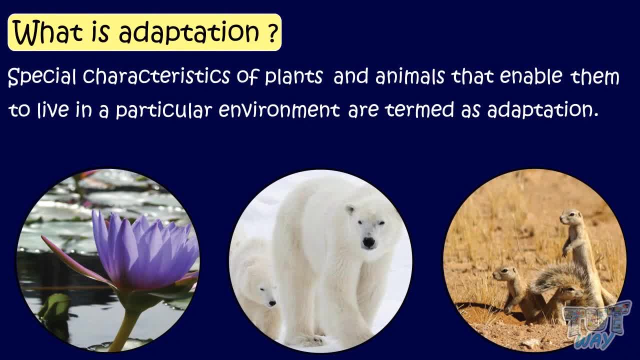 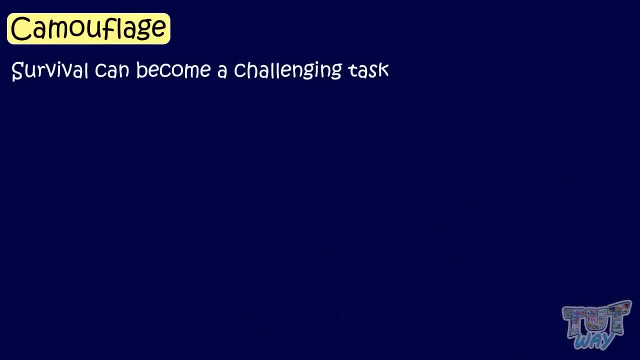 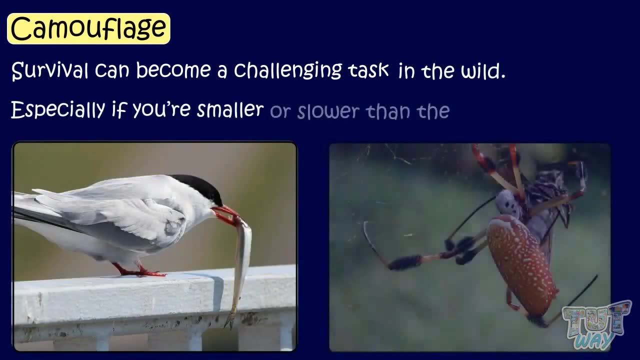 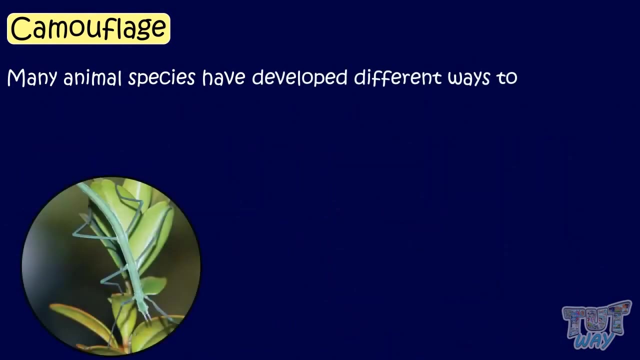 of adaptations. Let's learn about a few of them. Camouflage Survival can become a challenging task in the wild, especially if you're smaller or slower than the possible predators. This is why many animal species have developed different ways to camouflage. that is, blending itself. 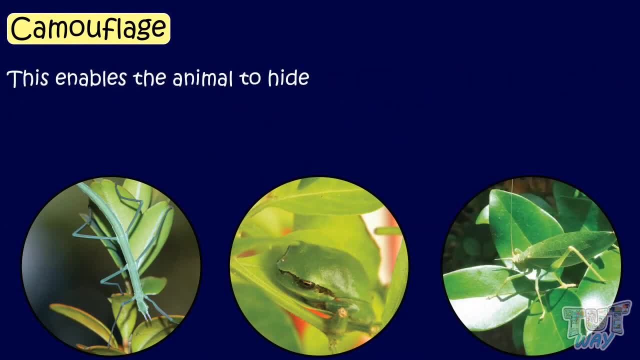 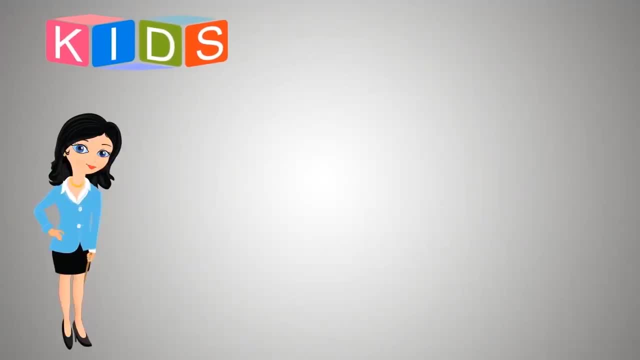 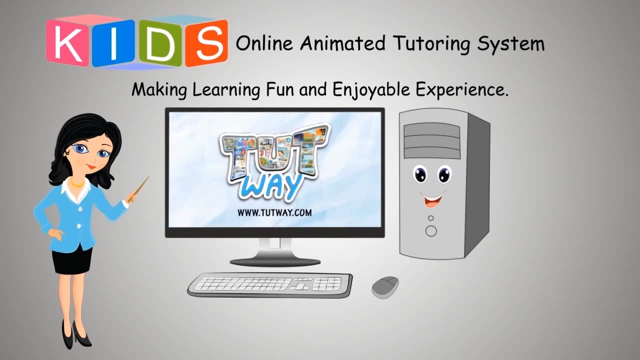 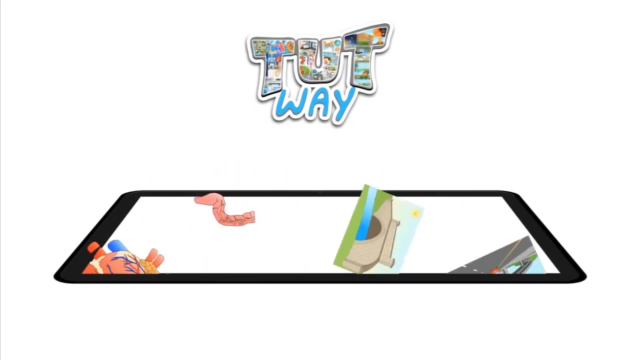 with the environment. Camouflage is a technique that allows animals to live in a particular environment. This enables the animal to hide from predators and also to catch up its prey. TootWay has thousands of animated videos on math, English and science to clear the core basics of 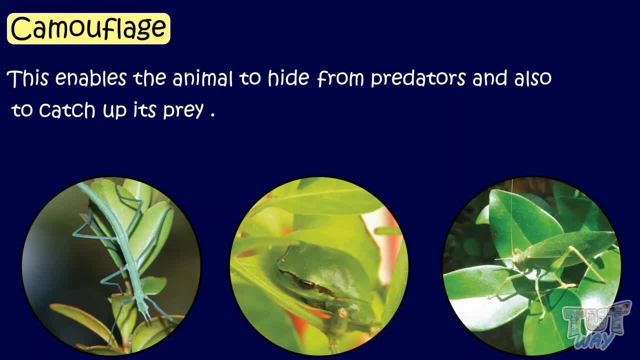 these subjects. TootWay has thousands of animated videos on math, English and science to clear the core basics of these subjects. Let's have a look at some examples. Let's learn how animal algae can start companion violence. This is a stick insect. It. 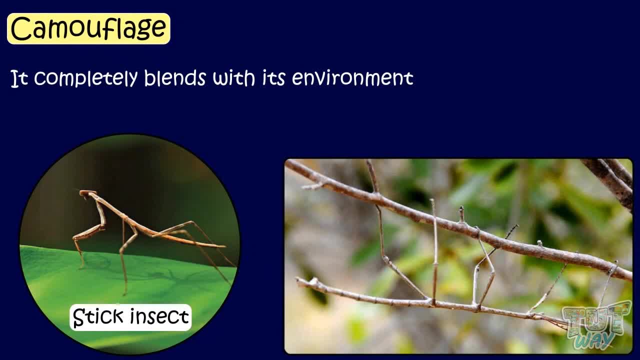 completely blends with its environment, That is, it looks like a stick itself. This way, it can hide from its predators and can catch its preys without making its preys getting to know of its presence. And can catch its prey, It can prey on prey And this kind of prey can detect and再來. 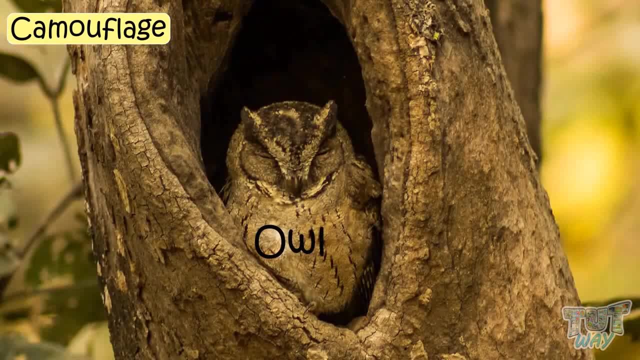 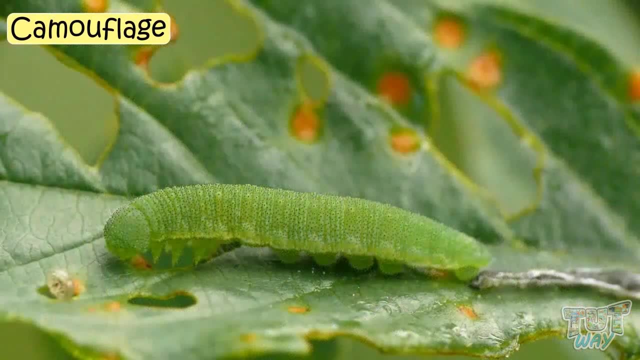 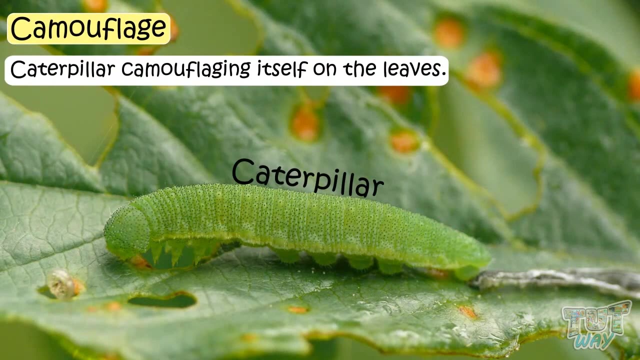 catch prey, And especially when statt prob посмотреть and be able to catch prey. Can it use a spirit camouflage? This is an owl. It completely blends itself with the trunk of a tree. This is a caterpillar camouflaging itself on the leaves. Here we have 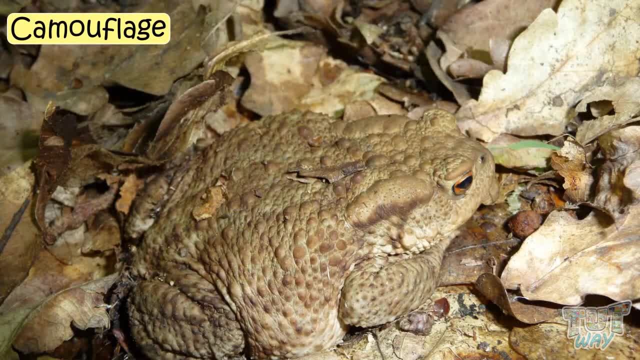 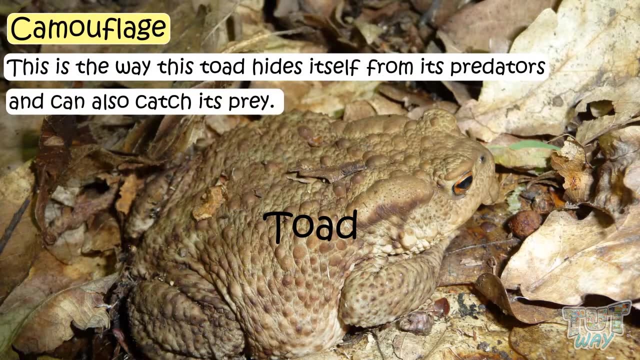 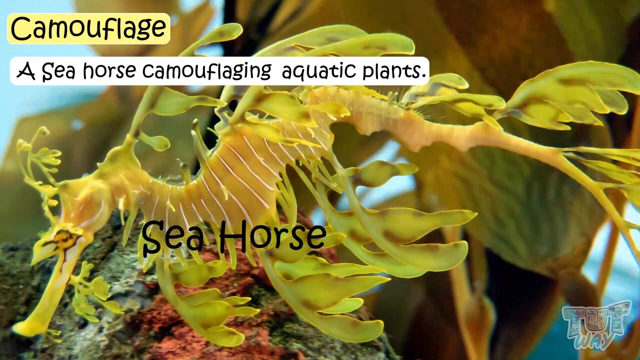 another example of camouflage. It's hard to find this toad in these leaves. Can you find them? So this is the way this toad hides itself from its predators and can also catch its prey. Here is a small seahorse camouflaging itself in aquatic plants. Here is another insect camouflaging. 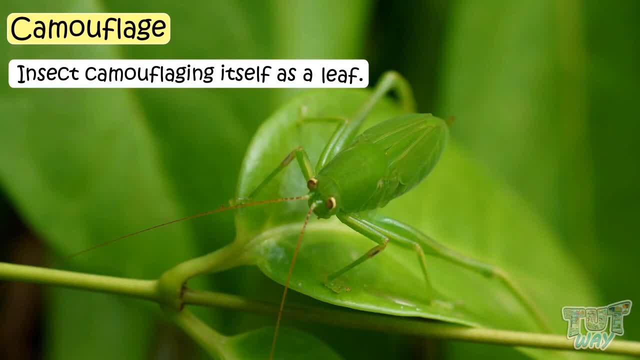 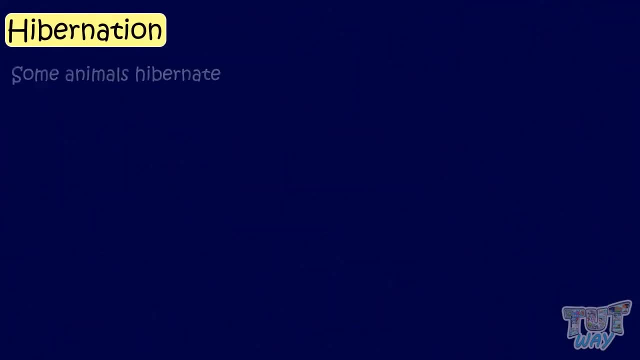 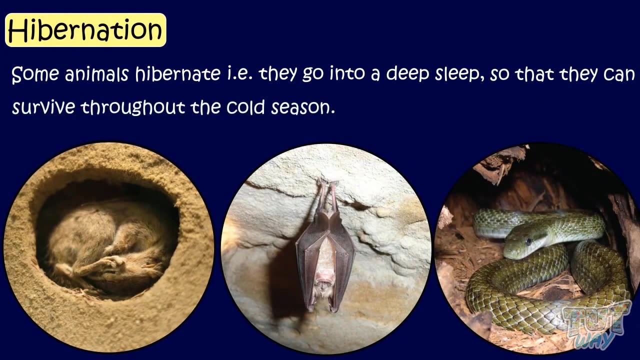 itself as a leaf. Now let's learn another type of adaptation in animals A: It is hibernation. Some animals hibernate, that is, go into deep sleep, so they can survive throughout the cold season, When the weather is freezing and the food is scarce. 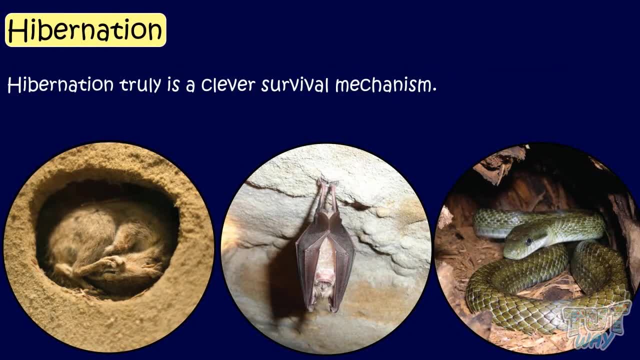 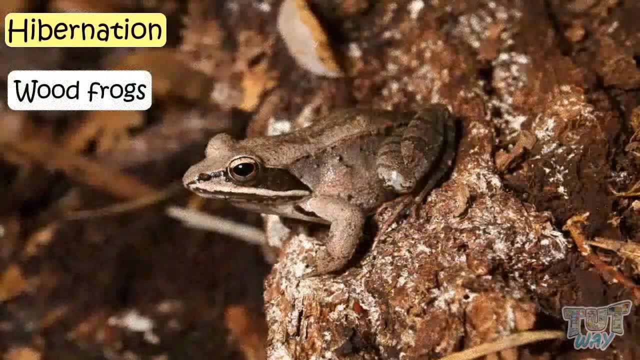 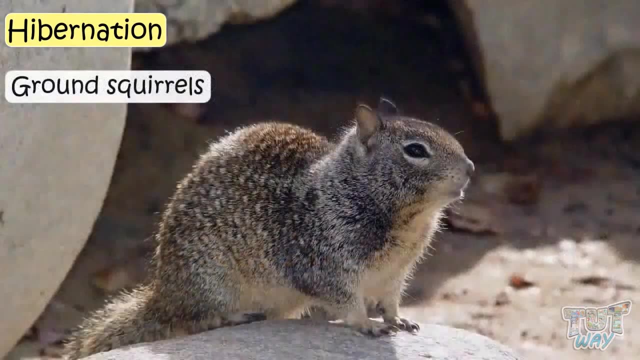 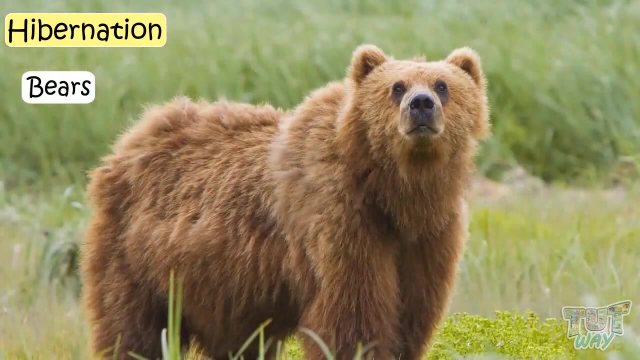 Hibernation truly is a clever survival mechanism. Now let's see some animals that can hibernate. Woodfrogs, Common poorwills, Ground squirrels, Hamsters, Bats, Bears, Garter, snakes And snails are some animals that hibernate. 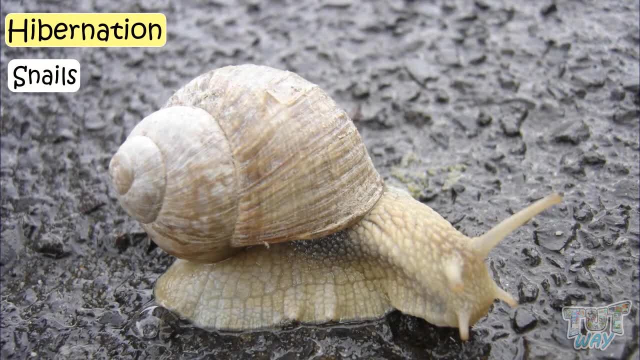 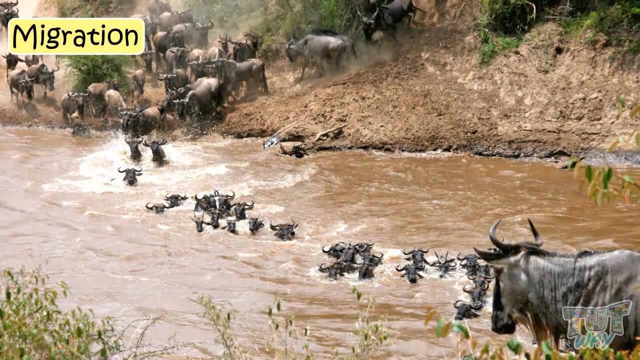 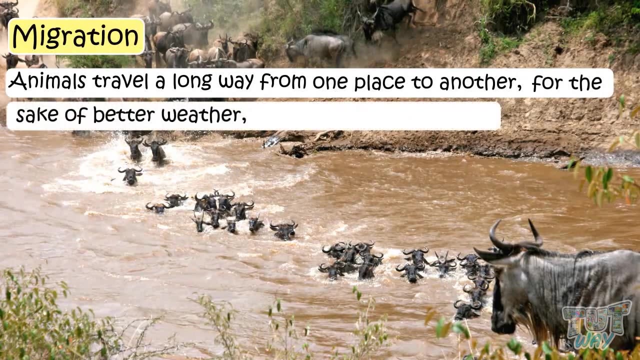 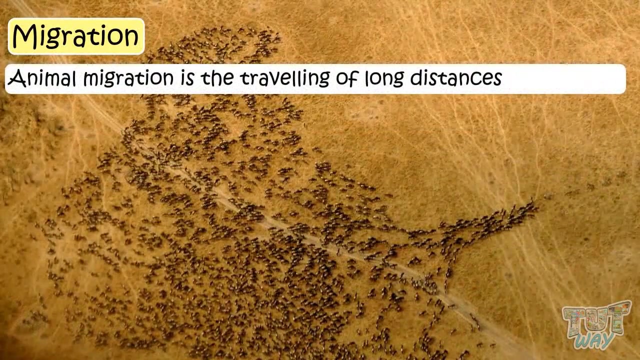 Now let's see another way of adaptation: Migration Migration: Animals travel a long way from one place to another for the sake of better weather, or breeding, or better food. Animal migration is the traveling of long distances in search of new habitat. It can be for breeding. 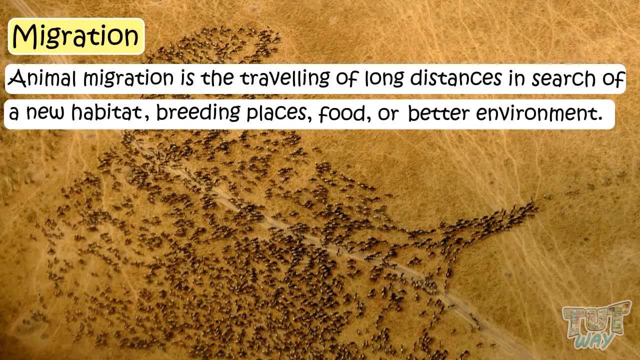 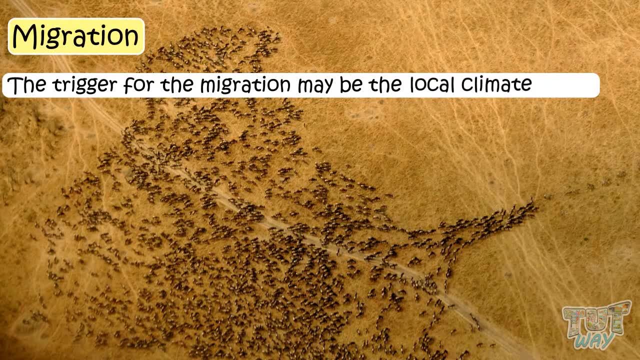 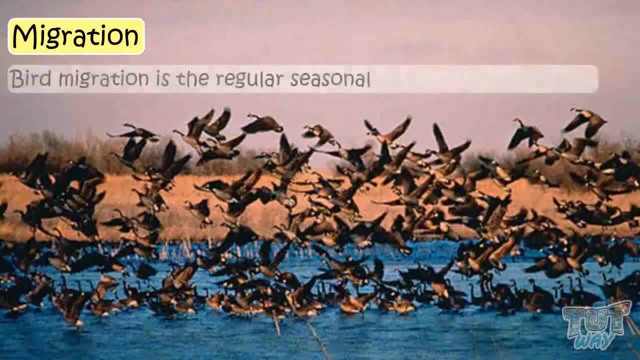 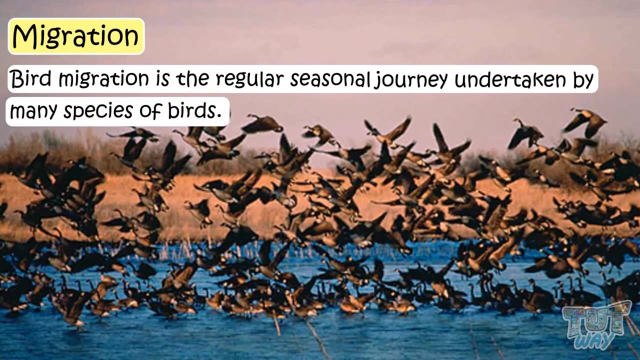 It can be for feeding, Or it can be for better environments or climates. The trigger for the migration. migration may be local climate, local availability of food or the season of the year. Bird migration is regular seasonal journeys undertaken by many species of birds. Bird movement include those: 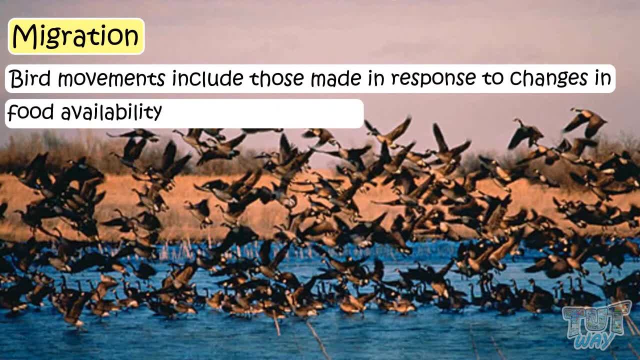 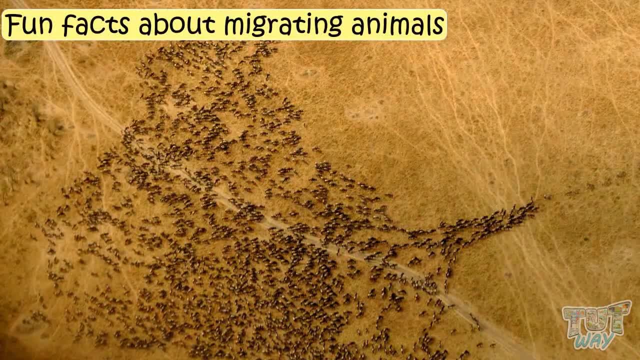 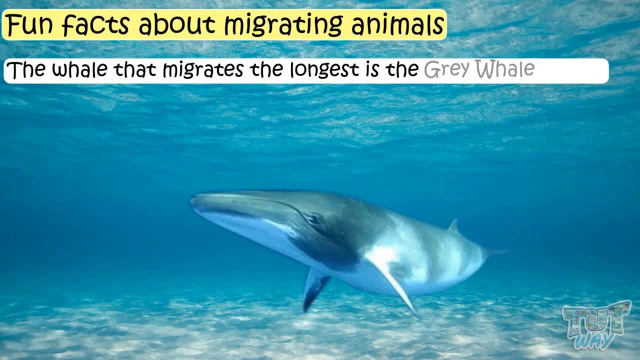 made in response to changes in food availability, habitat or weather. Now let's learn some fun facts about the migrating animals. The whale that migrates the longest is the gray whale, which migrates about 12,500 miles. The insect that migrates the longest is the desert locust.